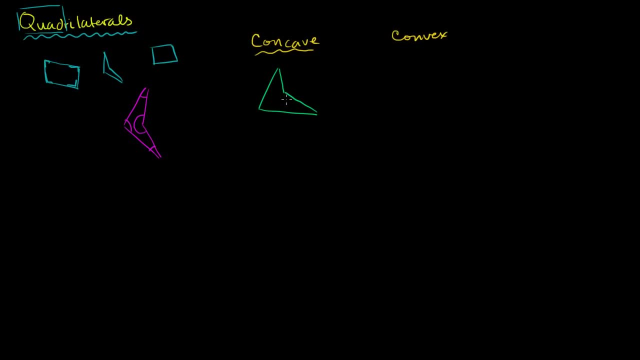 is that it has an interior angle that is larger than 180 degrees. So, for example, this interior angle right over here is larger than 180 degrees. It's an interesting proof. Maybe I'll do a video. It's actually a pretty simple proof. 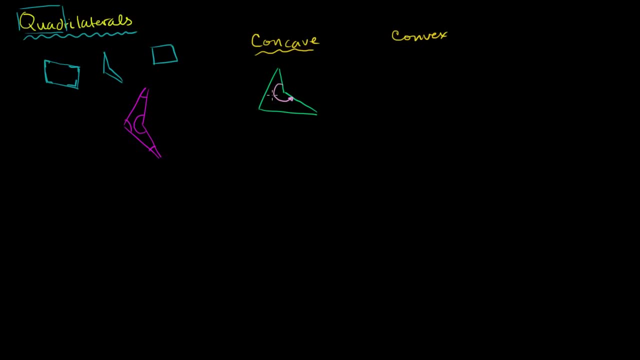 to show that if you have a concave quadrilateral, if at least one of the interior angles has a measure larger than 180 degrees, then none of the sides can be parallel to each other. The other type of quadrilateral you can imagine is when all of the interior angles 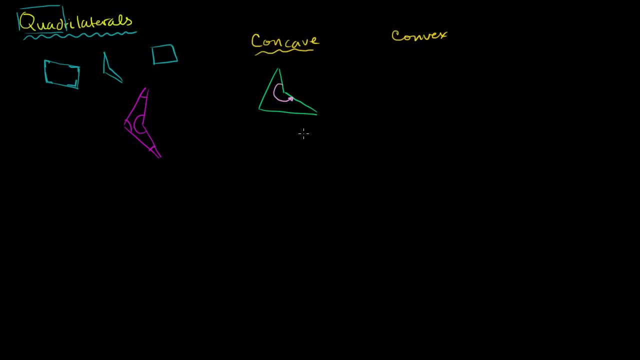 are less than 180 degrees, And you might say, wait, what happens at 180 degrees? Well, if this angle was 180 degrees, then these wouldn't be two different sides, It would just be one side and that would look like a triangle. 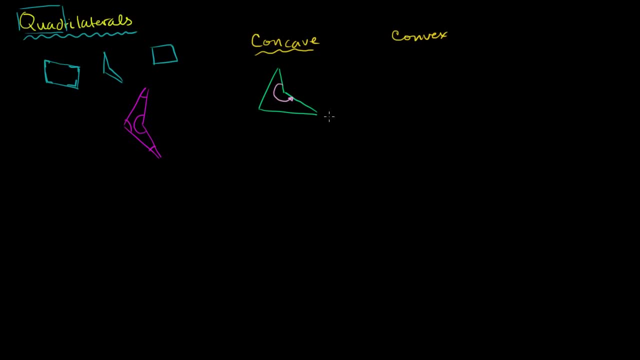 But if all of the interior angles are less than 180, then you are dealing with a convex quadrilateral. So this convex quadrilateral would involve that one and that one over there. So this right over here is what a convex quadrilateral could look like: four points, four sides, four angles. 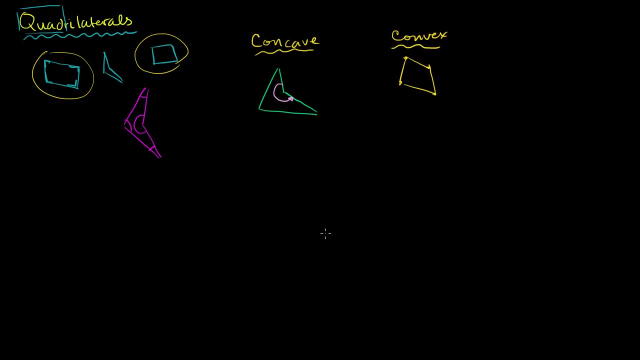 Now, within convex quadrilaterals there are some other interesting categorizations. So now we're just going to focus on convex quadrilaterals. So that's going to be all of the space over here. So one type of convex quadrilateral is a trapezoid. 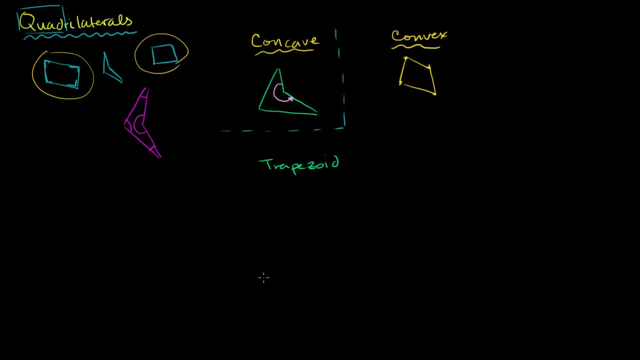 And a trapezoid is a convex quadrilateral And sometimes the definition here is a little bit different. people will use different definitions. So some people will say a trapezoid is a quadrilateral that has exactly two sides that are parallel to each other. 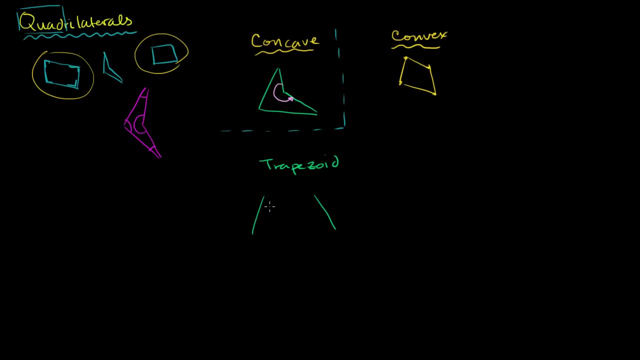 So, for example, they would say that this right over here is 80 degrees A trapezoid where this side is parallel to that side. If I give it some letters here, if I call this trapezoid ABCD. 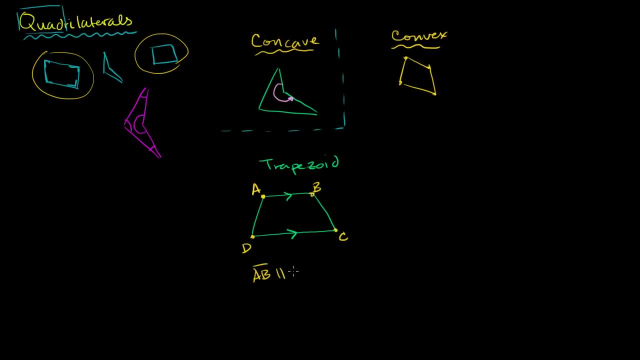 we could say that segment AB is parallel to segment DC And because of that we know that this is a trapezoid. Now I said that the definition is a little fuzzy because some people say you can have exactly one pair of parallel sides. 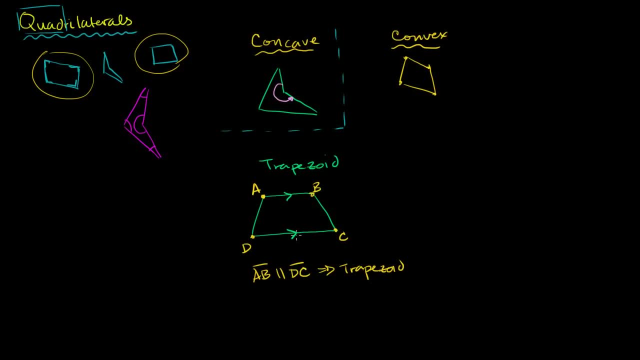 But some people say at least one pair of parallel sides. So if you use the original definition- and that's the kind of thing that most people are referring to when they say a trapezoid- exactly one pair of parallel sides, it might be something like this: 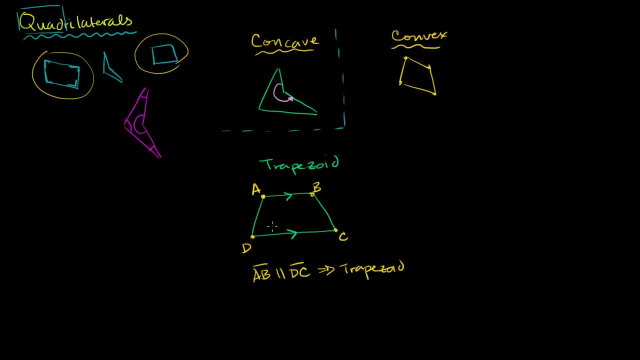 But if you use the broader definition of at least one pair of parallel sides, then maybe this could also be considered a trapezoid. So you have one pair of parallel sides like that, and then you have another pair of parallel sides like that. 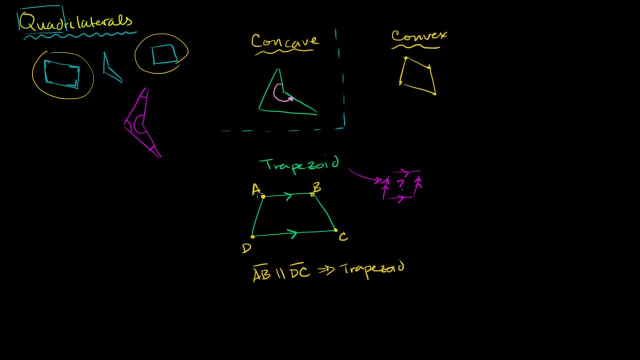 So this is a question mark where it comes to a trapezoid. A trapezoid is definitely this thing here, where you have exactly one pair of parallel sides. Depending on people's definition, this may or may not be a trapezoid. 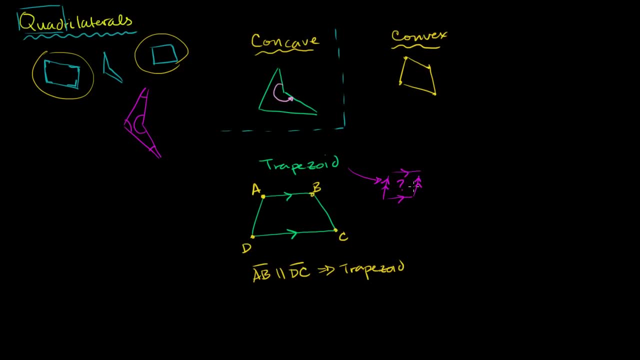 If you say it's exactly one pair of parallel sides, this is not a trapezoid, because it has two pairs. If you say at least one pair of parallel sides, then this is a trapezoid. So I'll put that in a little question mark there. 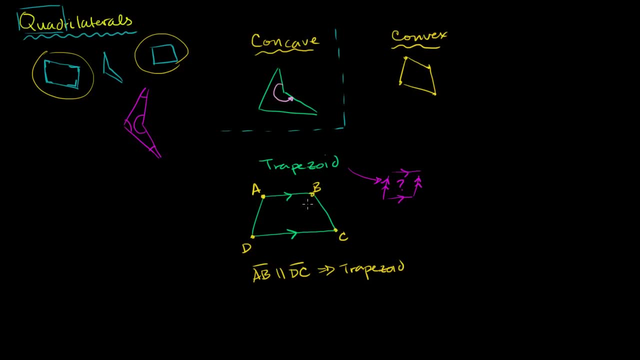 But there is a name for this, regardless of your definition of what a trapezoid is. If you have a quadrilateral with two pairs of parallel sides, you are then dealing with a parallelogram, So the one thing that you definitely can call this. 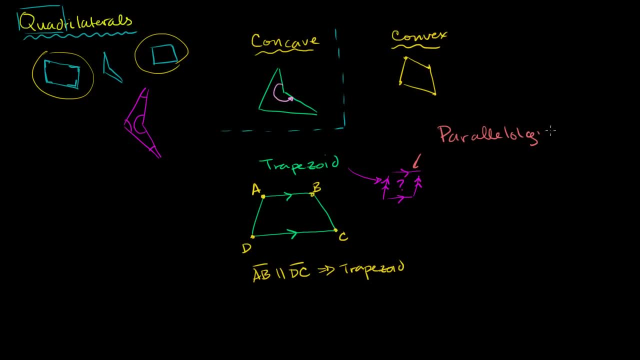 is a parallelogram. Parallelogram and I'll just draw it a little bit bigger, So it's a quadrilateral. and if I have two pairs of parallel sides, or the opposite sides are parallel, So that side is parallel to that side. 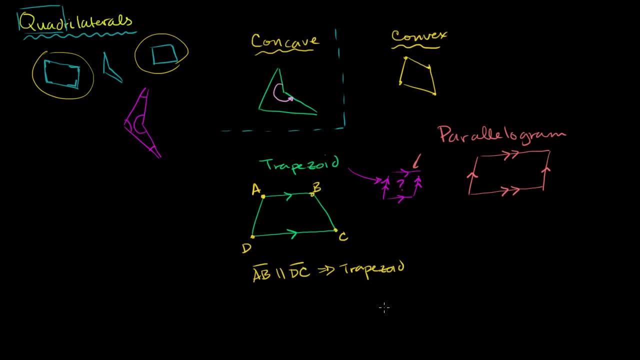 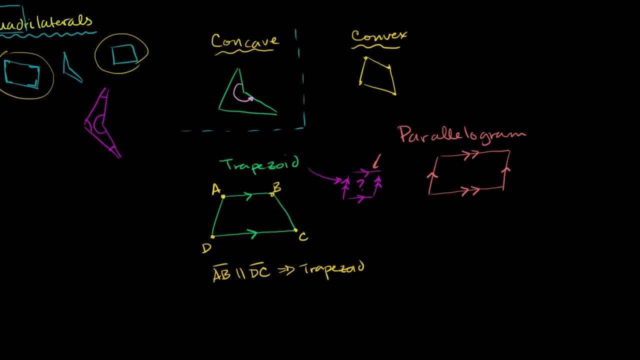 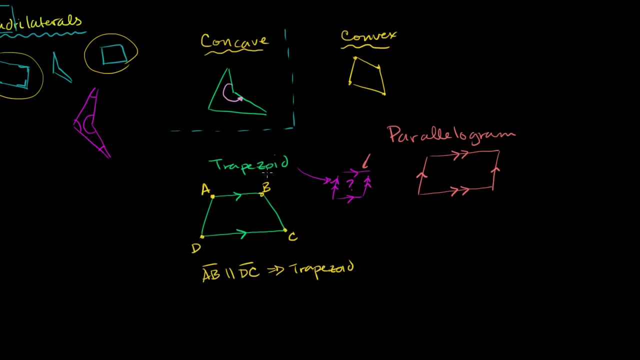 and then this side is parallel to that side. there You're dealing with a parallelogram, And then parallelograms can be subdivided even further. If the four angles in a parallelogram are all right angles, you're dealing with a rectangle. 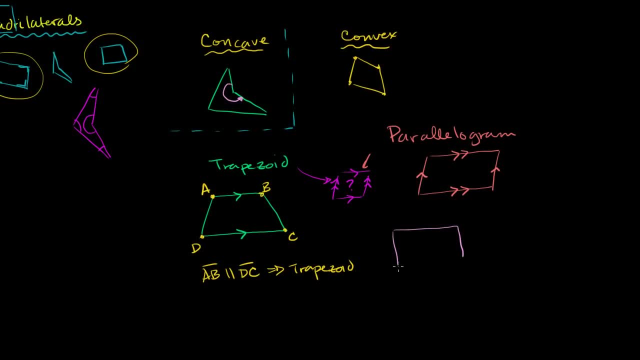 So let me draw one like that. So from parallelograms, this is all in the parallelogram universe what I'm drawing right over here, This is all the parallelogram universe. So the parallelogram tells me that opposite sides. 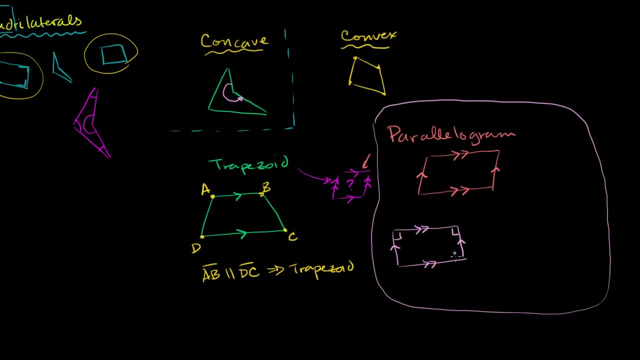 are parallel. And then if we know that all four angles are 90 degrees and we've proven in previous videos how to figure out the sum of the interior angles of any polygon, and using that same method you could say that the sum of the interior angles 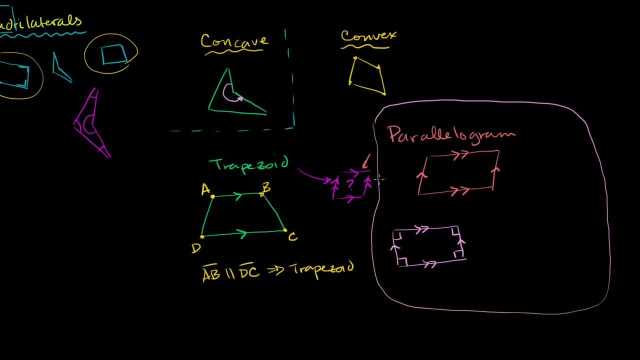 of any quadrilateral is actually 360 degrees, And you see that in this special case as well, but maybe we'll prove it in a separate video. But this right over here we would call a rectangle Parallelogram: opposite sides, parallel. 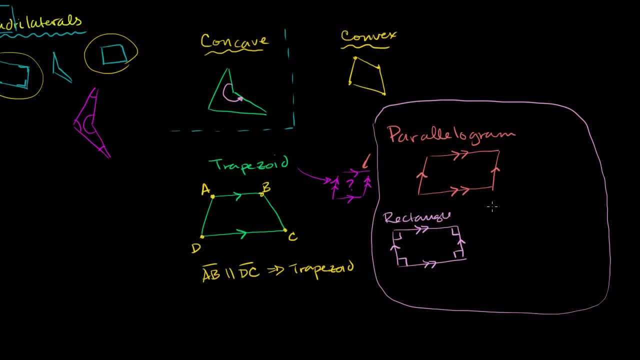 and we have four right angles. Now, if we have a parallelogram where we don't necessarily have four right angles, but we do have the length of all the sides being equal, then we're dealing with a rhombus. So let me draw it like that. 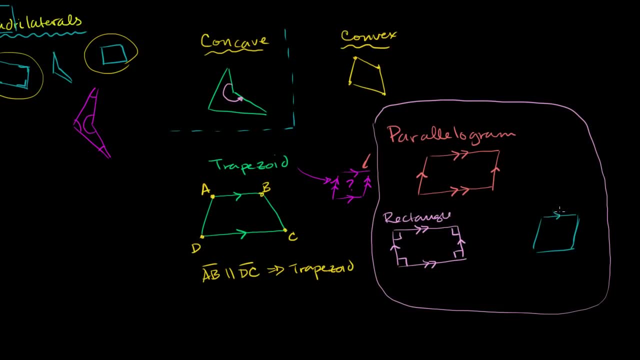 So it's a parallelogram. This is a parallelogram, So that side is parallel to that side, This side is parallel to that side, And we also know that all four sides have equal length, So this side's length is equal to that side's length. 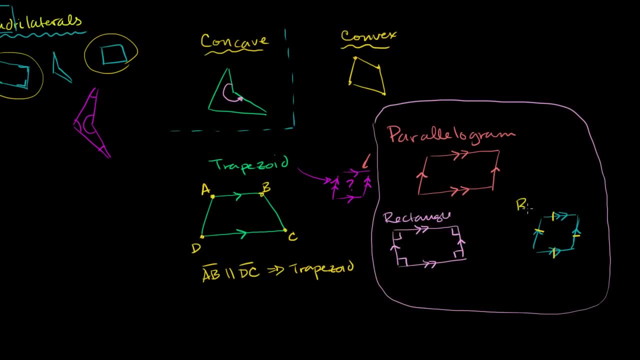 which is equal to that sides' length, which is equal to that side's length. Then we are dealing with a rhombus. So one way to view it: all rhombi are parallelograms, All rectangles are parallelograms. 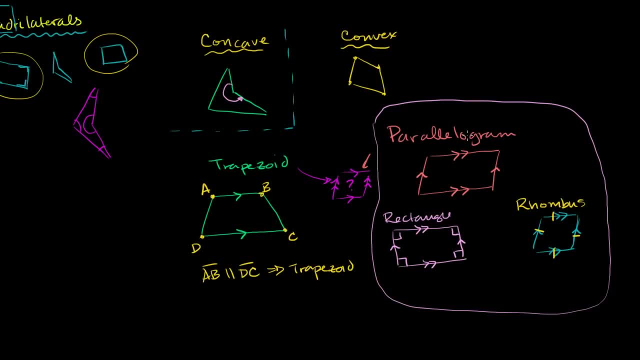 All parallelograms. you cannot assume to be rectangles. All parallelograms. you cannot assume to be rhombi. Now, something can be both a rectangle and a rhombus. So let's say that this is the universe of rectangles, So the universe of rectangles. 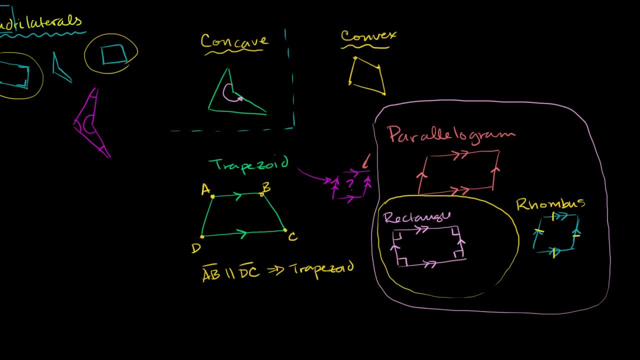 I'll draw a little bit of a Venn diagram. here is that set of shapes, And the universe of rhombi is this set of shapes right over here. So what would it look like? Well, you would have four right angles. 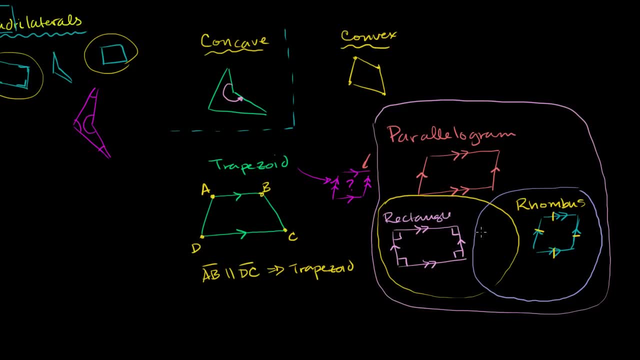 and they would all have the same length. So it would look like this. So it would definitely be a parallelogram. It would be a parallelogram Four right angles And all the sides would have the same length. This is probably the first of the shapes that you learned. 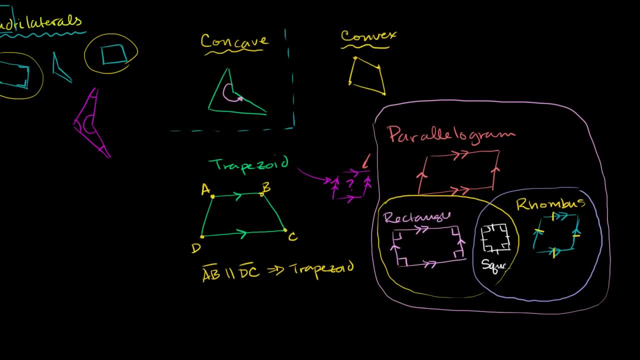 or one of the first shapes. This is clearly a square, So all squares are both rhombi, they can also be considered a rhombus, and they can also be considered a rectangle, and they can also be considered a parallelogram.